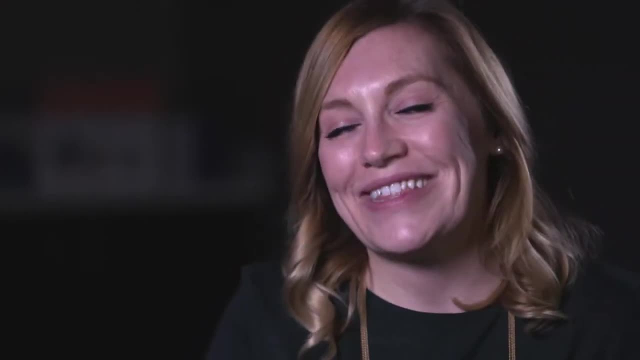 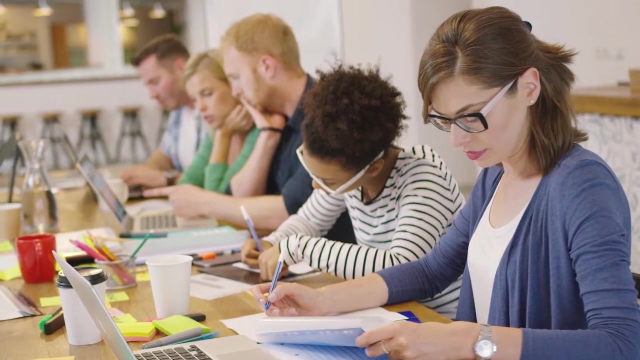 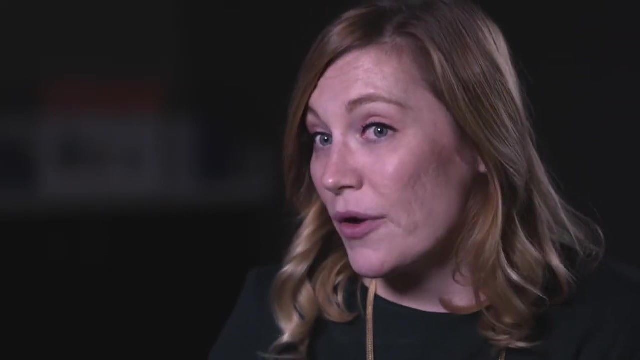 differently than I do, And so learning how to articulate those things really clearly has become super important, because if I'm not clear, they're not going to be able to navigate the process. So I go back and I meet with each department while they develop PD and they develop. 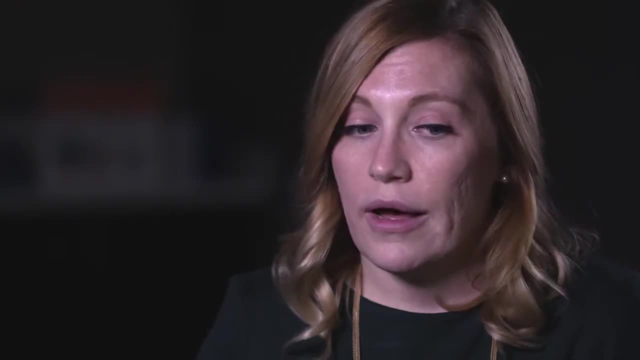 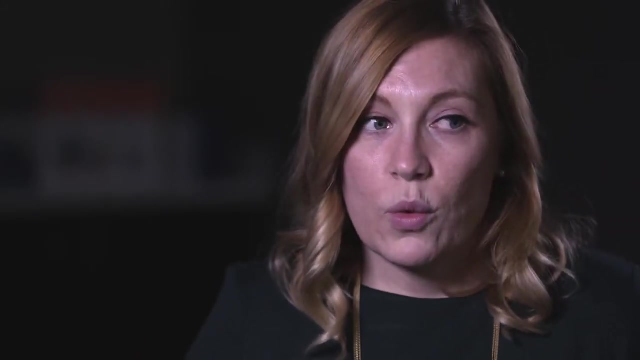 their goals and give feedback as to, yes, this will work, no, this won't. But it is very much a partnership. So every single department in my building, as much as we were working to achieve the same goal, they all did it differently. 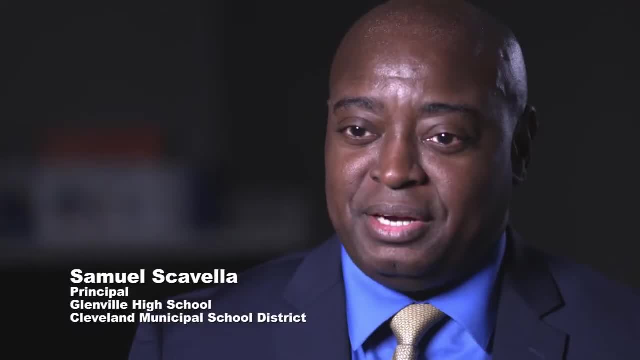 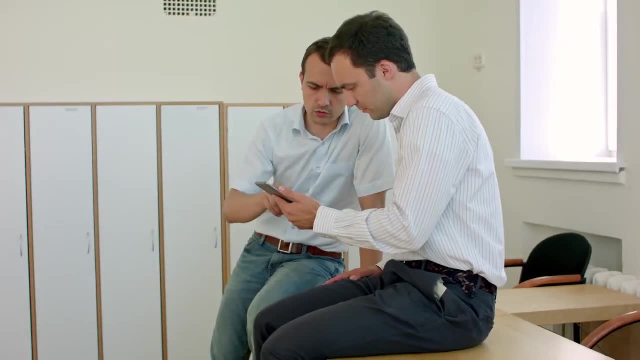 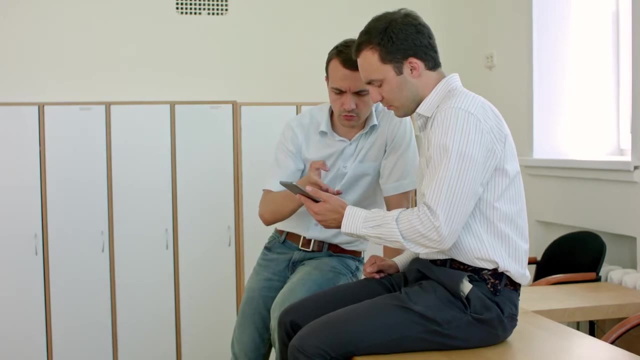 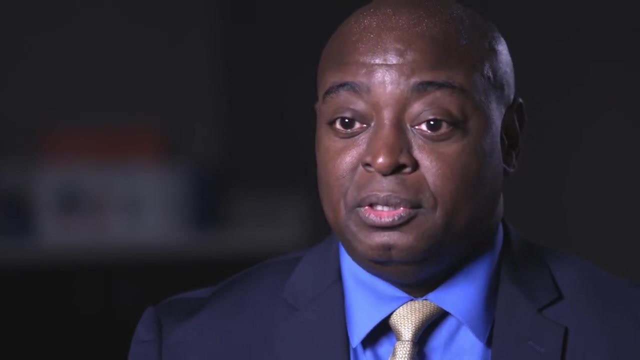 And that shift between when principals were managers and when we started having to be instructional leaders. we had to change how we conducted and offered professional development, And it was a total collaborative effort. Everyone had their roles. Everyone knew exactly what they were required to do or expected to do And the ones that didn't. we spelled it out. 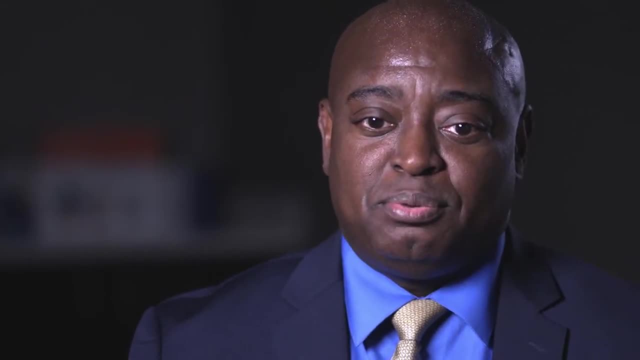 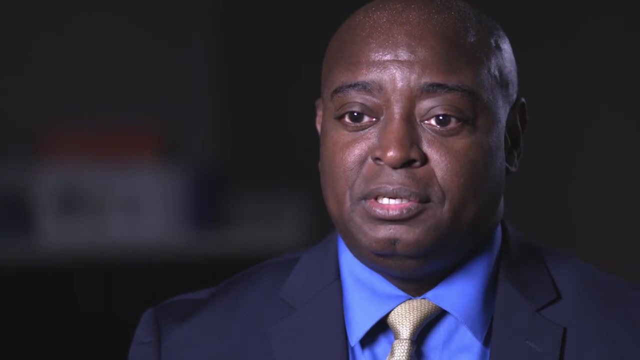 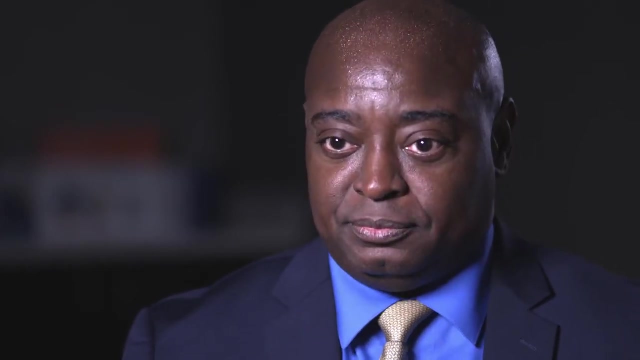 for them, And so, in leading that work, it was important for me to become the lead learner, for me to participate in all of the professional development activities that were going along, And I would, as I provide some, you know, I would be in there learning right alongside. 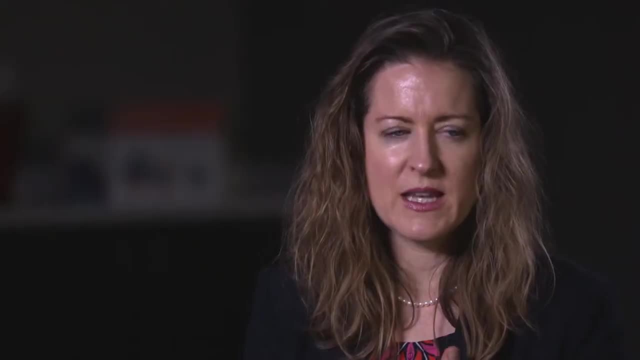 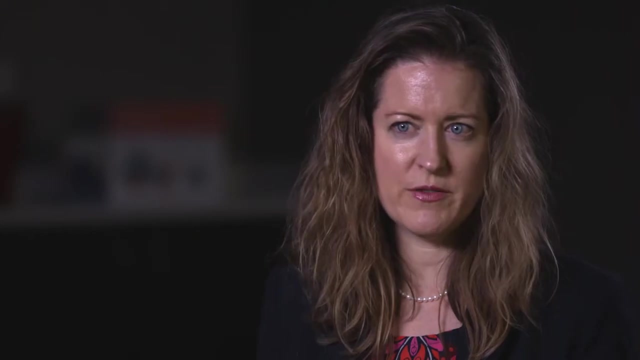 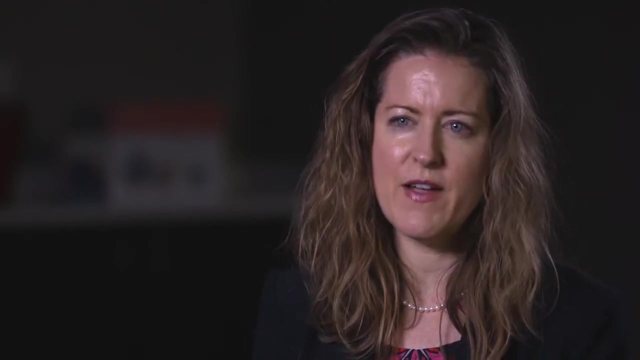 my teachers A priority for me to set conditions where teachers can rise into leadership roles and where I am present and supportive, But not the one who's talking all the time in a meeting, for example. So, and you know, in the five years that I've been in this building, we've definitely seen 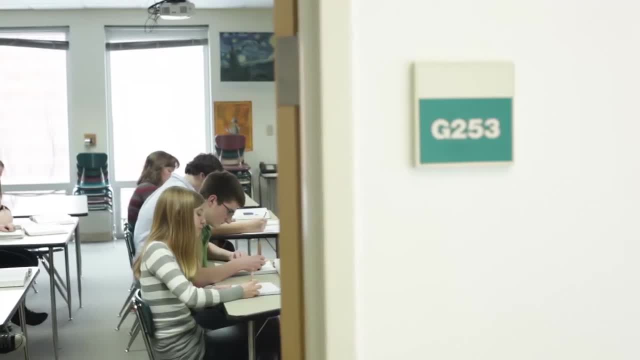 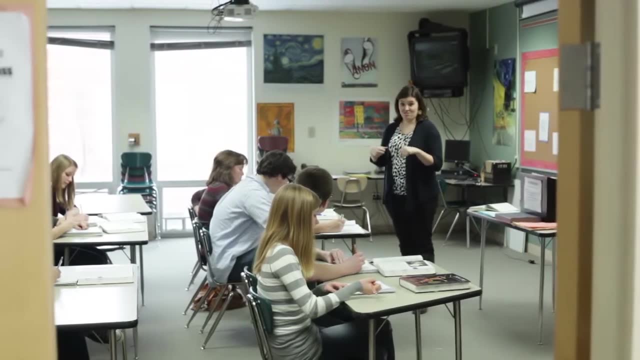 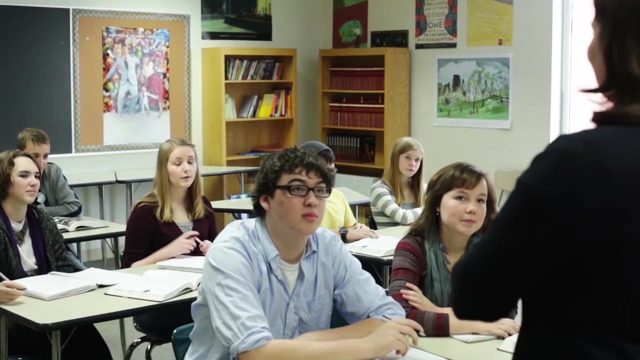 an increase in that And I think that the ownership over what happens is far enriched by me doing that And part of that. you know how do I cultivate. that is about looking for a work life balance. looking for well, what am I trying to get out of work? 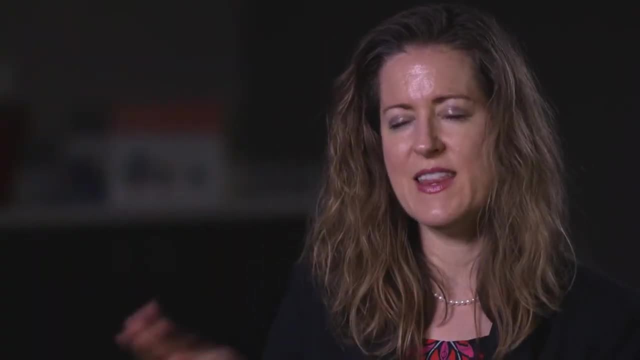 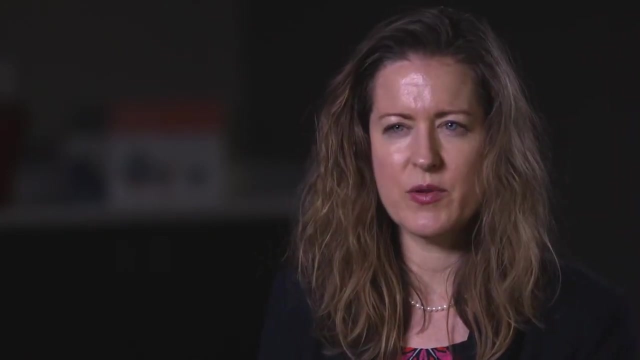 What am I trying to get out of being a principal And really getting the I as far away from that as possible? You know not needing it to be about what I accomplish, what my rating is, what people think of the work I do as building leader.